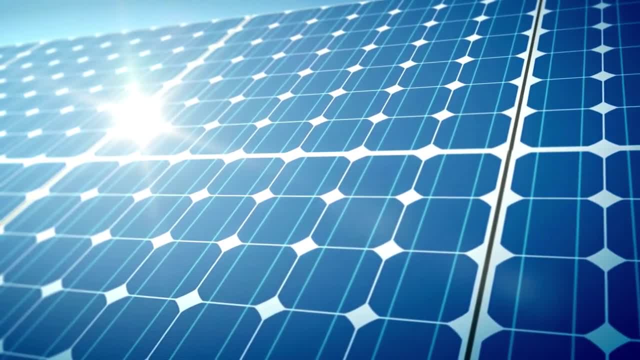 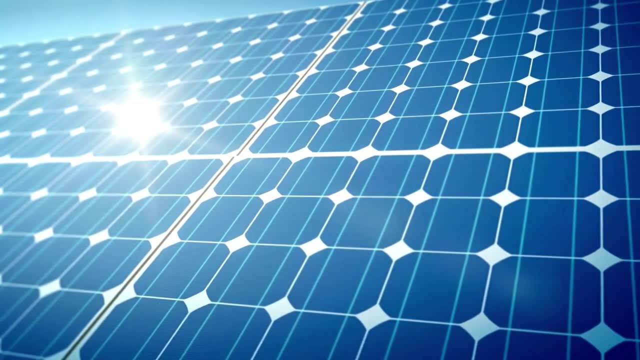 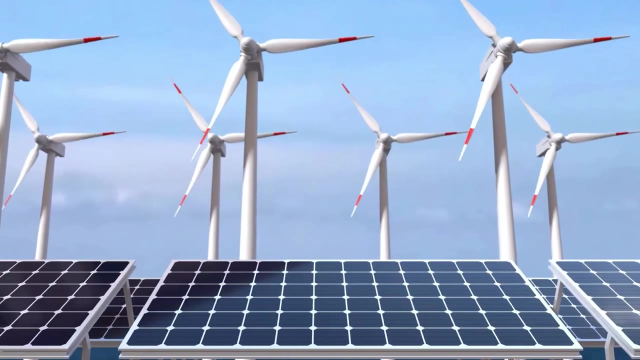 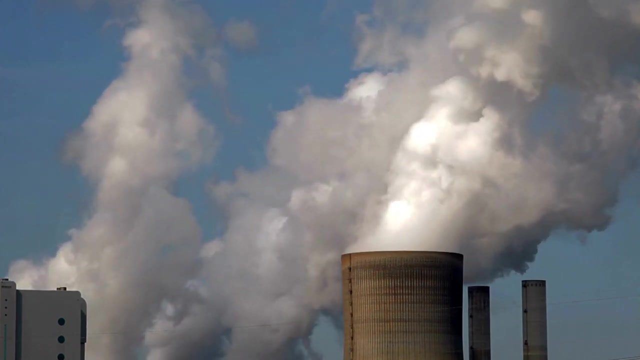 towards improving or protecting human life, For example, volcanologists or geologists who study volcanoes closely, monitor active ones and create early warning systems to evacuate towns before any volcanic eruptions. Many geologists work in the resource industry, finding new places or developing new ways to extract minerals or energy without harming the environment. 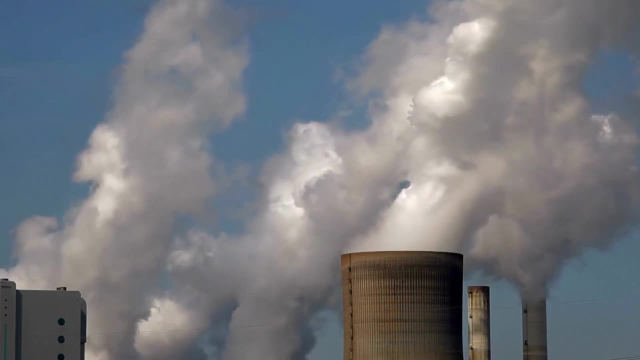 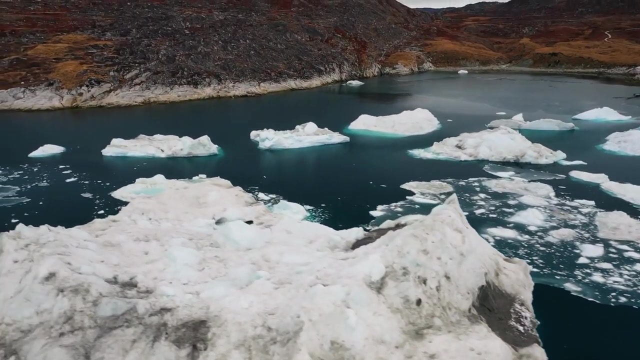 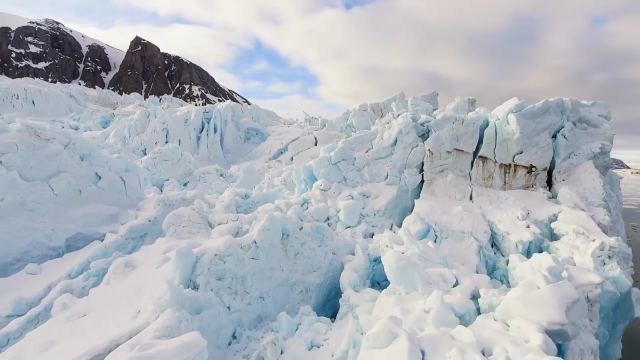 Others assess hazards to human life like volcanic eruptions, as was mentioned earlier, slope failures, massive floods and structural damage from earthquakes. Biologists interested in the evolution of life on Earth work closely with geologists in looking at the rock records to find fossils and footprints of organisms that are now extinct. Today we are 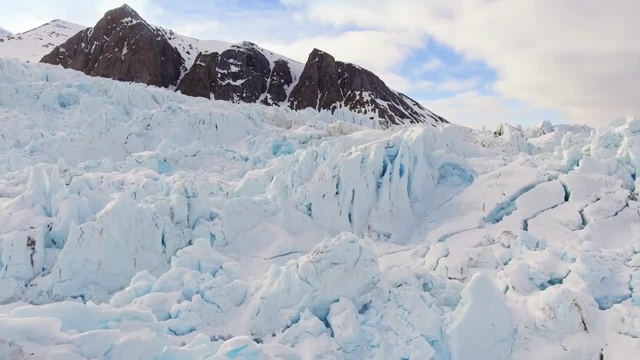 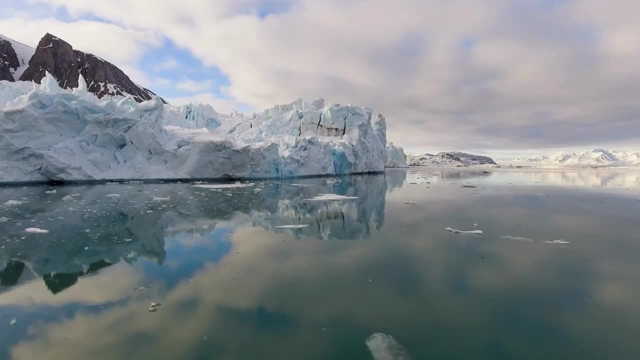 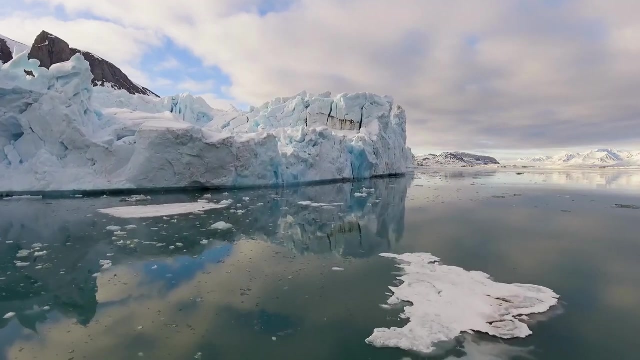 concerned about climate change. Many geologists are working to learn about the past climates of Earth and how they have changed across time. This historical geology information is valuable to understand how our current climate is changing and what the results might be. So, as you can see, 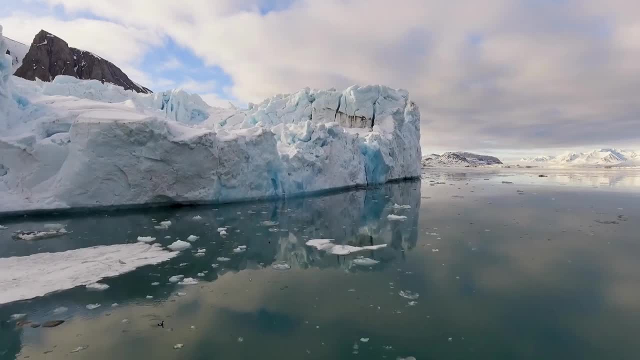 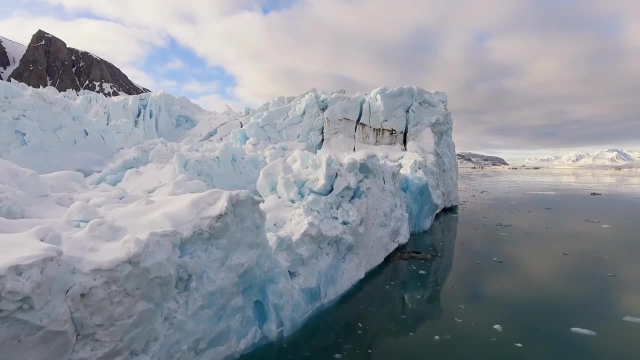 geology is not just about looking at rocks. It is rich and multifaceted, and there are many other things that can be done to help us understand the future of our planet. So, depending on your interests, you might focus on soil, minerals, water, natural resources or the. 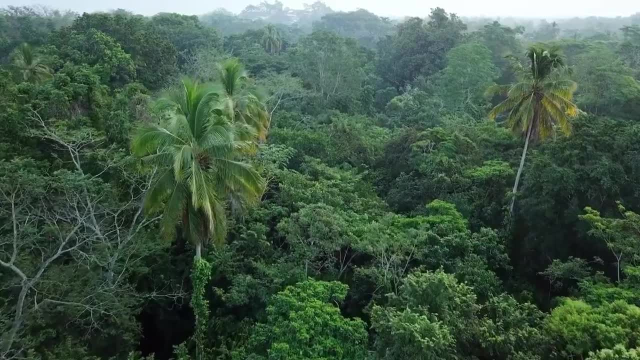 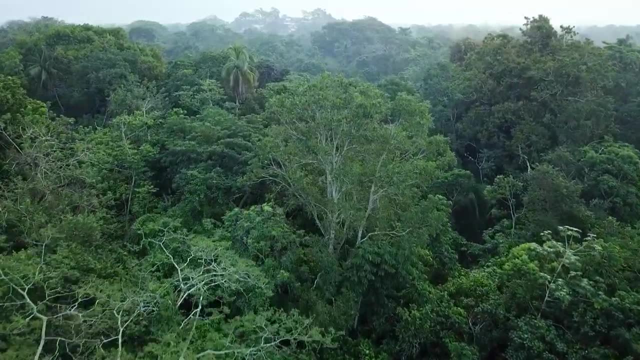 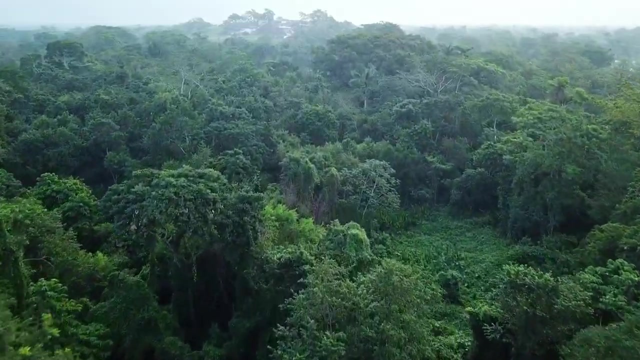 atmosphere. There are certain skills one must possess to be a geologist. One keen observation skills. Geologists must have a sharp sense of observation to quickly and effectively notice key features of the environment, survey sites and determine what samples are needed for further. 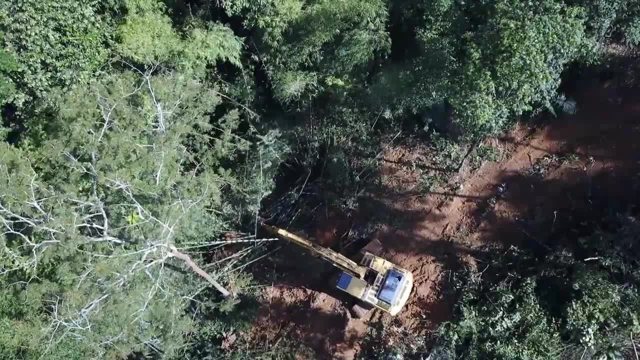 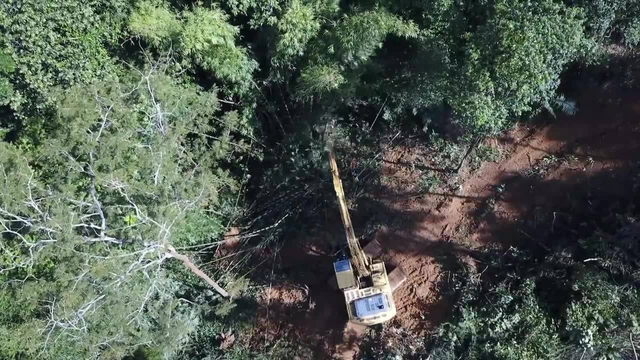 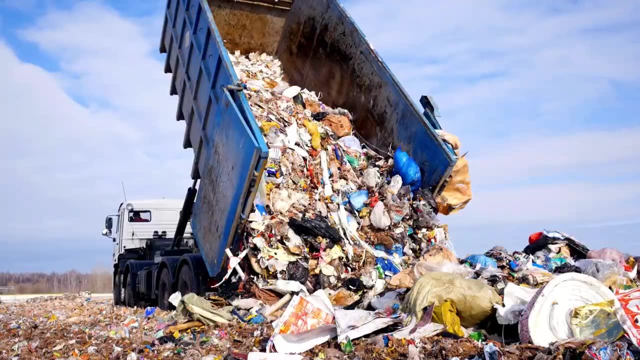 investigation. Two: analytical abilities: Geologists need a solid background in math, physics and biology to formulate questions based on the scientific method and conduct effective experimentation and investigation. Three: comfortable with technology. Geologists need to be proficient in operating and maintaining. 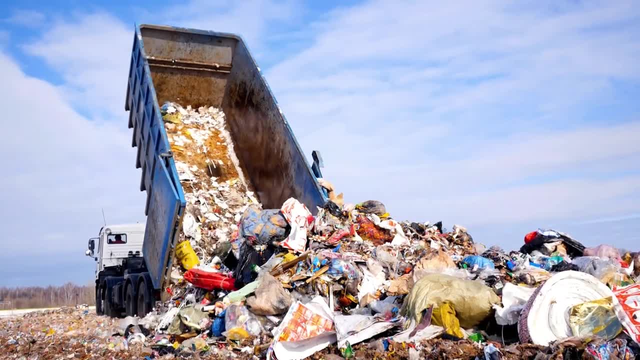 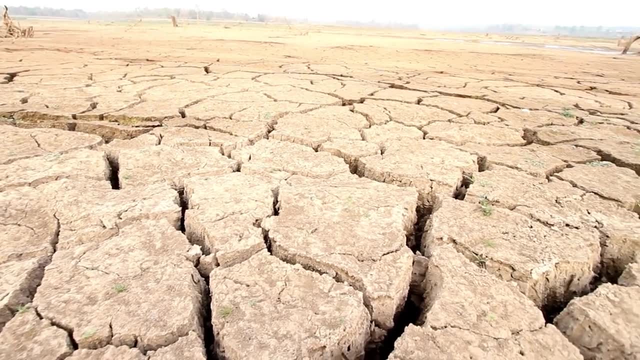 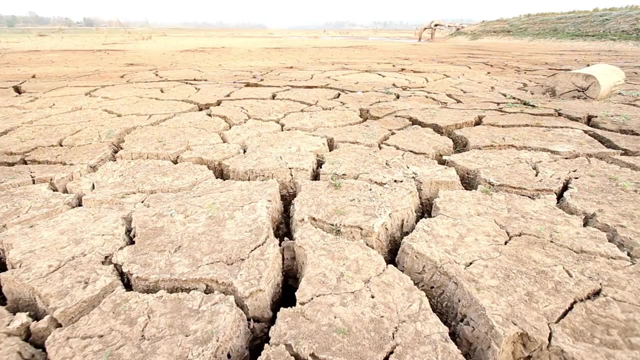 lab machinery, such as microscopes and advanced computer programs, as many spend more time in the lab than in the field. And four communication skills. Geologists must have strong written and verbal communication skills to complete grant applications, work with a variety of clients and present their work at professional meetings. The minimum training required to become a geologist is a four-year degree from a university specializing in earth science. In addition to core geology courses, a typical curriculum would include at least some entry-level interdisciplinary coursework in physics, chemistry and math. This training is a little different than any other course.